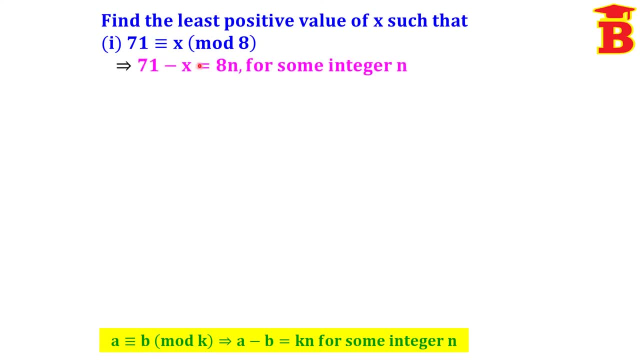 That is 71 minus X equal to. Here the mod number is 8.. So we can write 8 N for some integer N. So this means 71 minus X is a multiple of 8.. Because we have 71 minus X equal to 8 into N, So 8 times any integer. 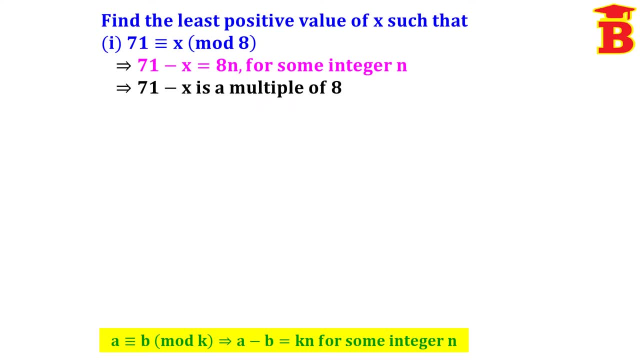 So we say that it is a multiple of 8.. Now the question is: we have to find the least positive value of X. So for that the easy method is: put X is equal to 1,, 2,, 3, etc. and check the answer. 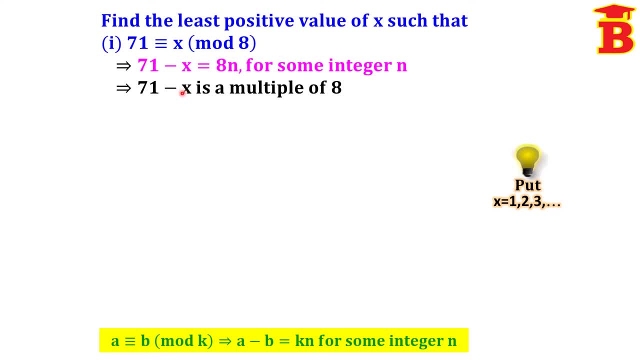 So if we take X is equal to 1,, 71 minus 1 is 70. It is not a multiple of 8.. Next, put X is equal to 2, we get 69. It is also not a multiple of 8.. 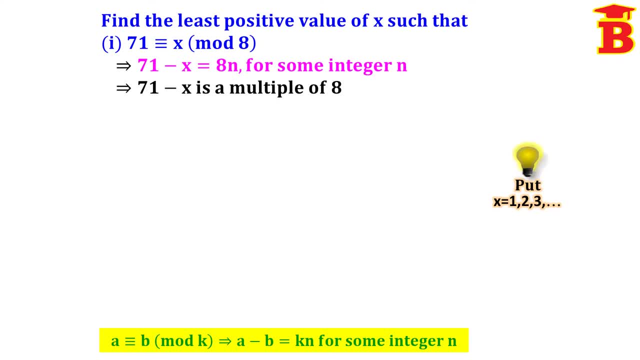 So like that, we have to check the number 1 by 1.. Here, if you put X is equal to 7, then we get 71 minus 7, that is 64.. 64 is a multiple of 8.. So therefore the answer is 7.. 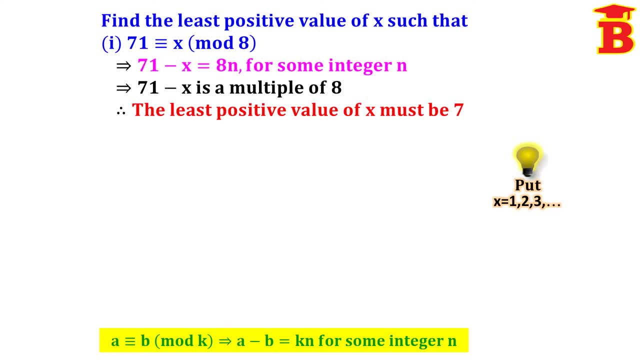 So the least positive value of X must be 7.. Similarly, next problem: Given 78 plus X is identical to 3 mod 5.. So arrange all the terms. left side, That means this: 3. take it to the left side, 78 plus X minus 7.. 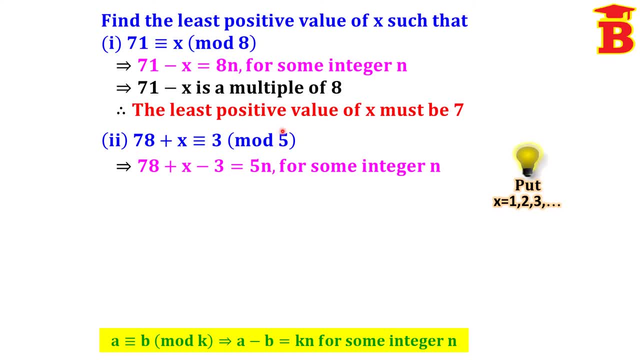 78 minus 3, equal to the mod number, is 5.. So we write 5n for some integer n. This left hand side, 78 minus 3, is 75 plus X is a multiple of 5.. Because right side we have 5n. 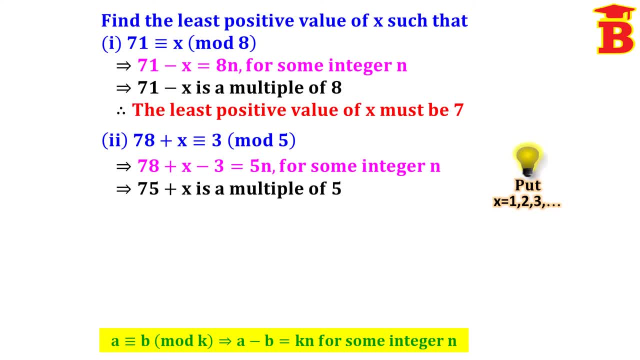 So 5 times any integer, So that we write it as multiple of 5.. Now if we put X is equal to 1,, then we get 75 plus 1, 76. It is not a multiple of 5.. Put X is equal to 2,, we get 77.. 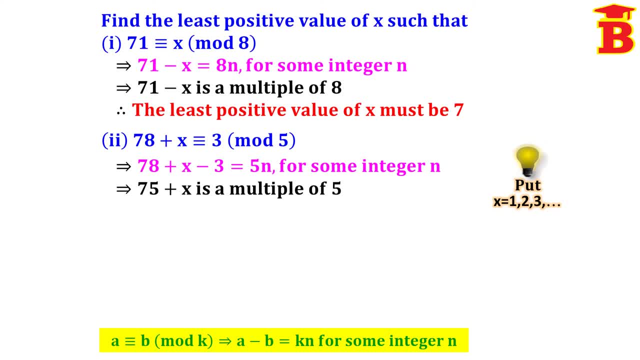 It is also not a multiple of 5.. So like that we have to check the number 1 by 1.. Here, if you put X is equal to 5, we get 75 plus 1.. So we write 75 plus 5, 80.. 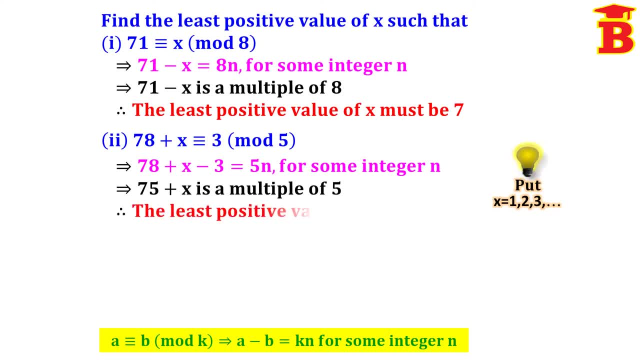 That is a multiple of 5.. Therefore, the least positive value of X must be 5.. Similarly, third sum 89 is identical to X plus 3 mod 4.. Arrange the terms left side. We get 89 minus of X plus 3, equal to 4n. 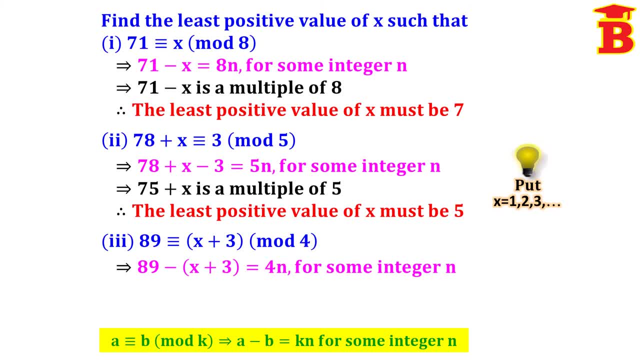 Here the mod number is 4.. So we write 4n for some integer n. Now left hand side, we get 89 minus 3 is 86 minus X Is a multiple of 4.. Because right side we have 4n. 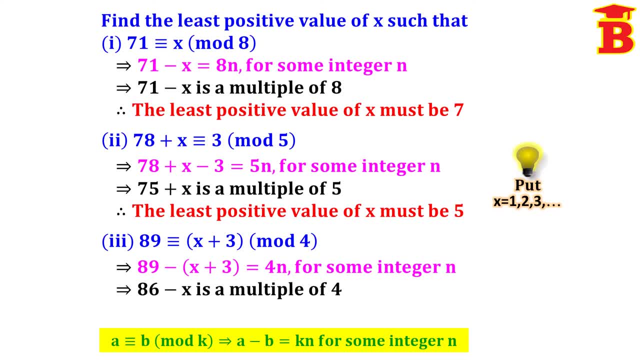 So it is a multiple of 4.. Now put X is equal to 1.. We get 86 minus 1, 85. It is not a multiple of 4.. Next we try the number 2.. Put X is equal to 2.. 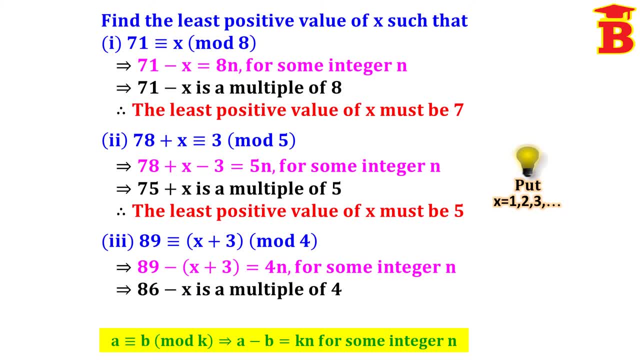 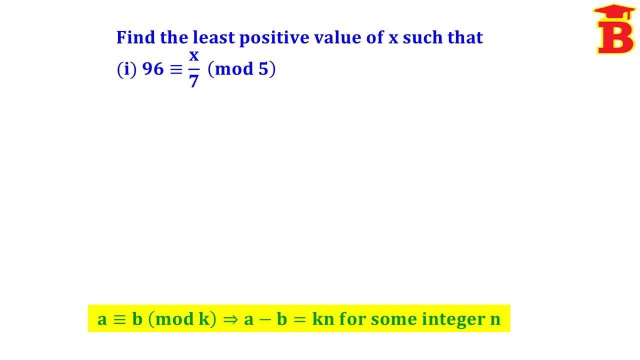 86 minus 2 is 84. It is a multiple of 4.. Therefore, the least positive value of X must be 2.. Similarly, let us see the next problem: Find the least positive value of X, Such that first equation 96, identical to X divided by 7 mod 5.. 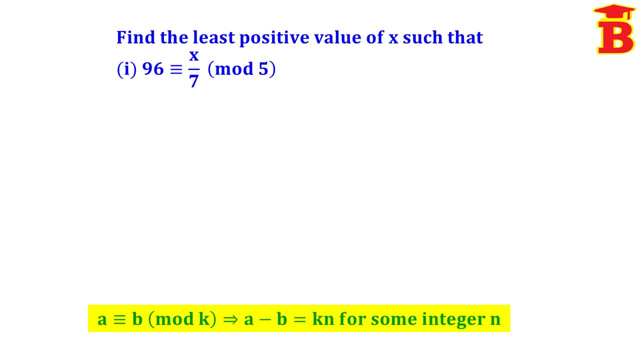 So here also same meaning. A is identical to B. mod K means We write A minus B. N is also equal to K, N For some integer n. So arrange the terms. left side: We get 96 minus X by 7. Equal to 5N. 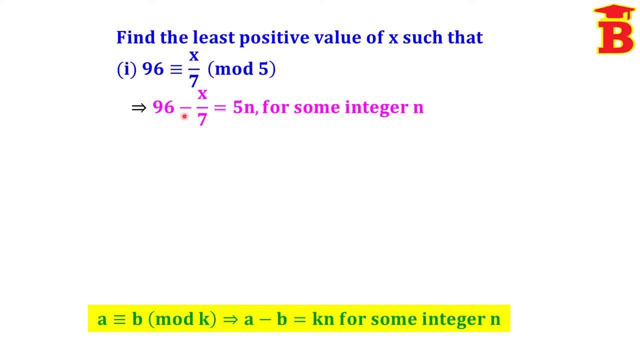 So this X by 7, take left side, We get 96 minus X by 7.. Here the mod number is 5.. So we write equal to 5N for some integer N, n. So this implies 96 minus x by 7 is a multiple of 5. Right side we have 5, n, So it is a. 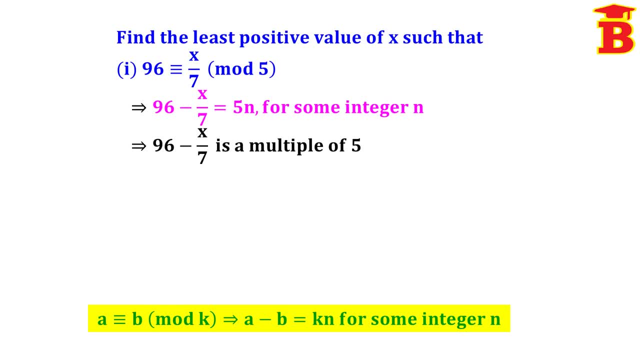 multiple of 5.. Now the question is: we have to find the least positive value of x. So we have to try. x is equal to 1,, 2,, 3, etc. And we have to check the given condition. 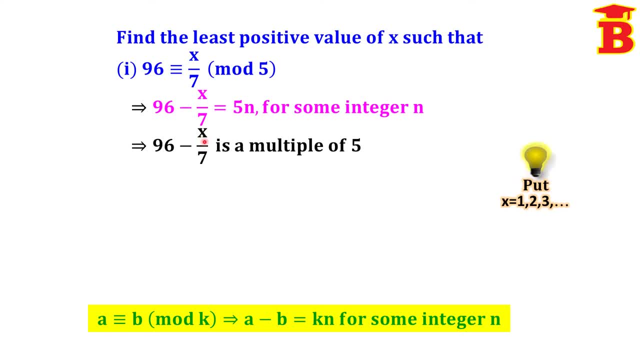 Here: if we take x is equal to 1, then we get 1 by 7. It is a fraction. So 96 minus 1 by 7 is a fraction number. So we cannot get multiple of 5. We have to get an integer. 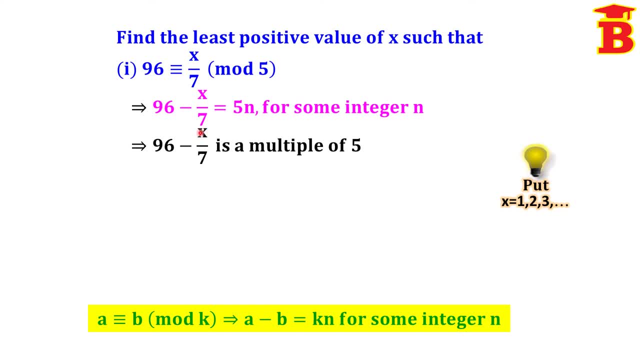 So that means we have to take: x is equal to 7.. Then only we can get 7 divided by 7, 1.. So now we can check this: If we take x is equal to 7, 7 divided by 7, 1. That is 96. 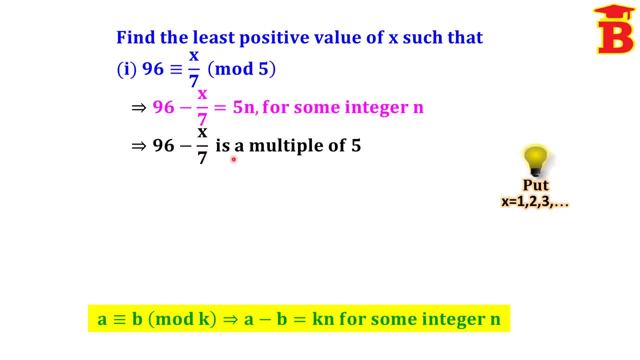 minus 1 is 95, which is a multiple of 5.. Therefore the x value is 7.. So this implies the least positive value of x must be 7.. Similarly, next problem, 5x, identical to 4, mod. 6.. Arrange the terms left side, That is 5x minus 4, equal to the.